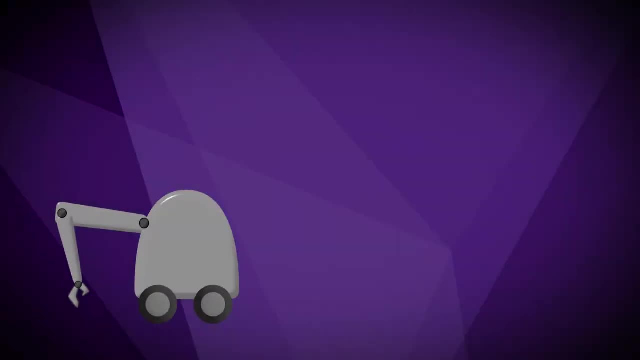 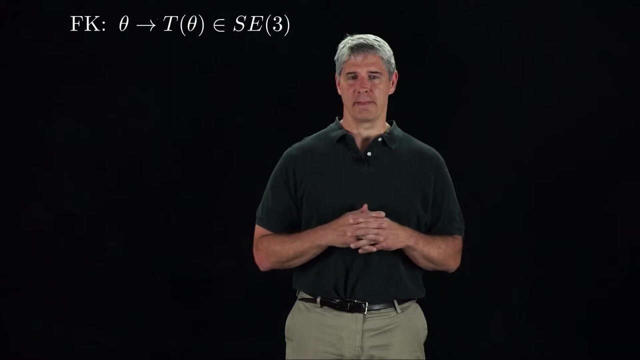 The forward kinematics maps the joint vector theta to the transformation matrix representing the configuration of the end effector. For simplicity, we will start instead with a coordinate-based forward kinematics where f of theta is a minimal set of coordinates describing the end effector configuration. Then the inverse kinematics problem is to find a joint vector. 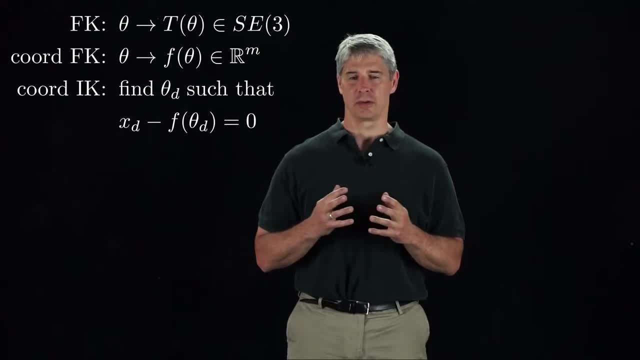 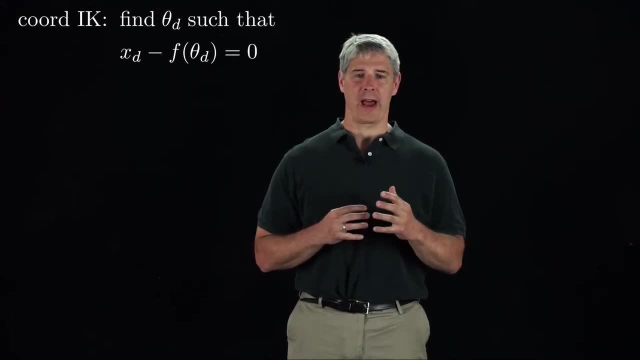 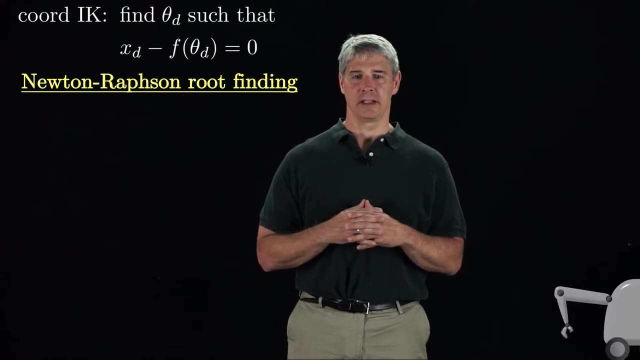 theta d satisfying xd minus f of theta d equals 0, where xd is the desired end effector configuration. To solve this problem, we will use the Newton-Raphson numerical root-finding method. In the case that theta and f of theta are scalars, the Newton-Raphson method can be illustrated easily. 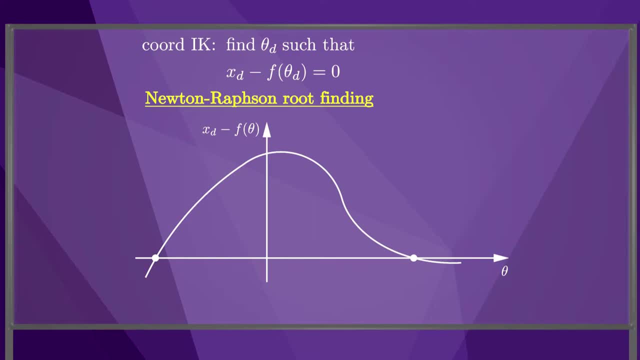 Here is a plot of the desired end effector position xd minus f of theta as a function of theta. The roots of this function correspond to joint values that solve the inverse kinematics. In this example, two values of theta solve the inverse kinematics. 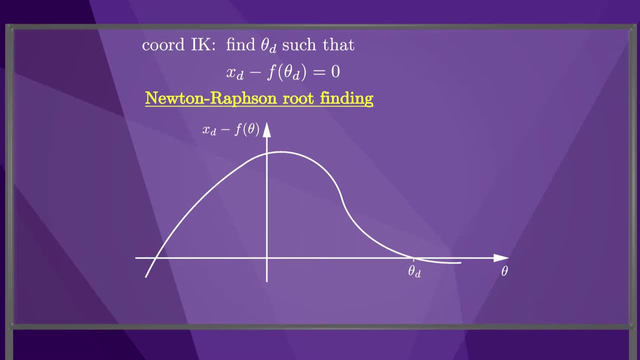 Now, with the benefit of hindsight, we designate one of the solutions as theta d. We also make an initial guess at the solution theta 0. At that guess we can calculate the value of xd minus f of theta. Since we know the forward kinematics f of theta, we can calculate. 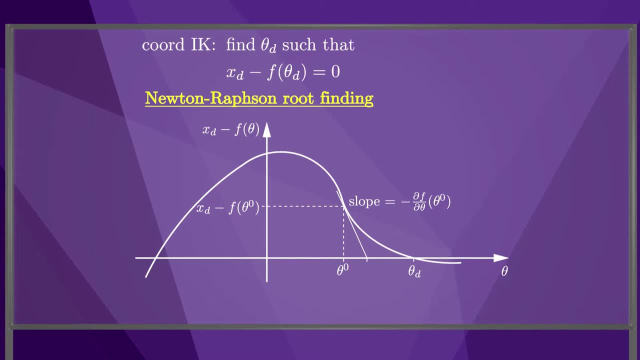 the slope of xd minus f of theta. If we extend the slope to where it crosses the theta axis, we get our new guess, theta 1.. The change delta theta in the guess is given by the expression in the figure. If the function xd minus f were linear, theta 1 would be an exact solution, Since it is not linear in. 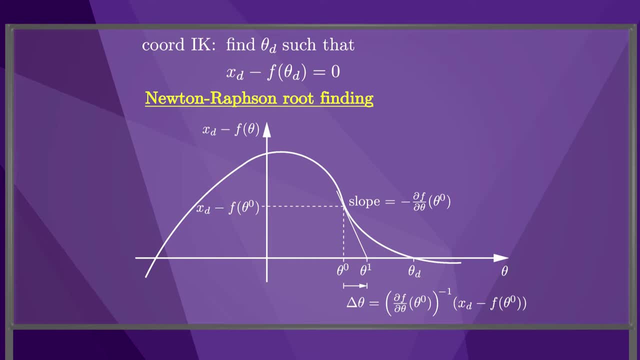 general, theta 1 is only closer to a solution, not an exact solution. Now we can repeat the process, getting a new guess, theta 2, and continue repeating until the sequence theta 0,, theta 1, theta 2, etc. converges to the solution theta d. 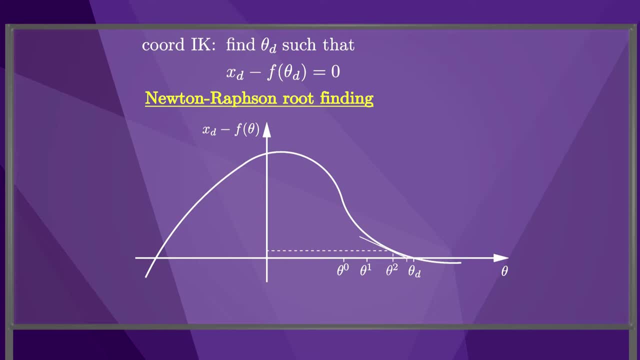 If our initial guess- theta 0- had been to the left of the plateau, we would have been able to calculate the value of xd minus f of theta and we would have been able to calculate the value of xd minus f of theta In general. the initial guess should be close to a solution to ensure that the process converges. 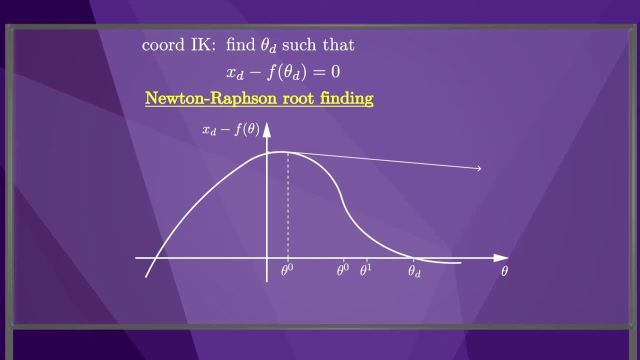 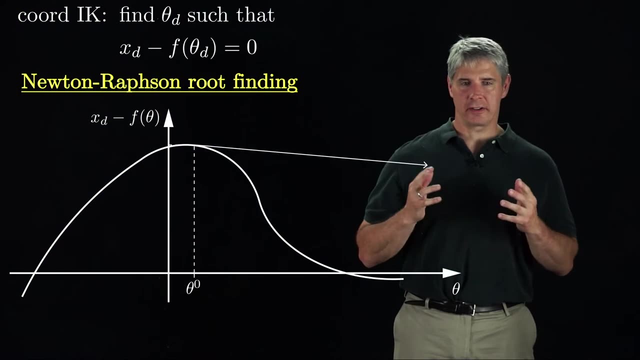 If the initial guess were near the top of the plateau, the calculated slope would have been small and the next iteration would be far away, where it may be difficult to converge to a solution To generalize the Newton-Raphson procedure to vectors of joints and endpoint coordinates. 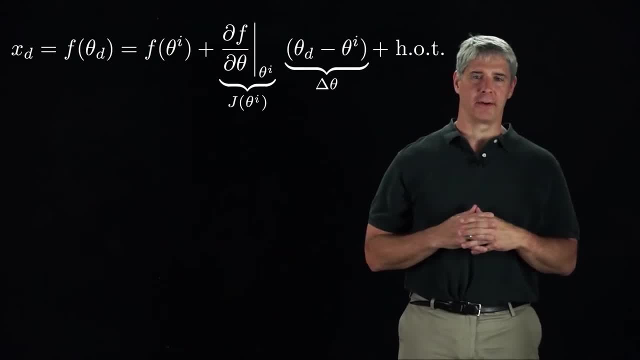 not just scalars. we can write the Taylor expansion of xd minus f of theta. We can write the Taylor expansion of xd minus f of theta In the definition letter seja. the organised function can Hm. We can put our operator here to factor a f account n as n. 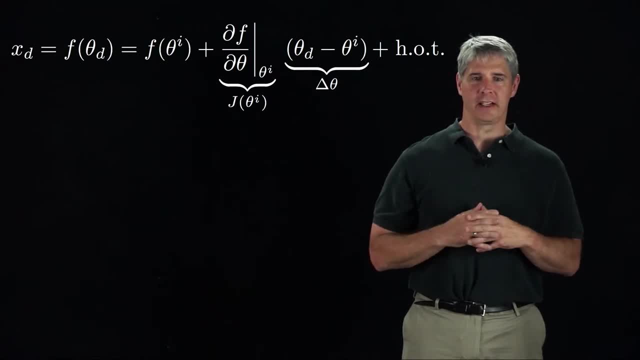 It is more efficient than thedoesn't change it. Now let's learn the expansion of the function f of theta around theta d. as shown here, f of theta is equal to f of theta i, where theta i is the current guess at the solution. 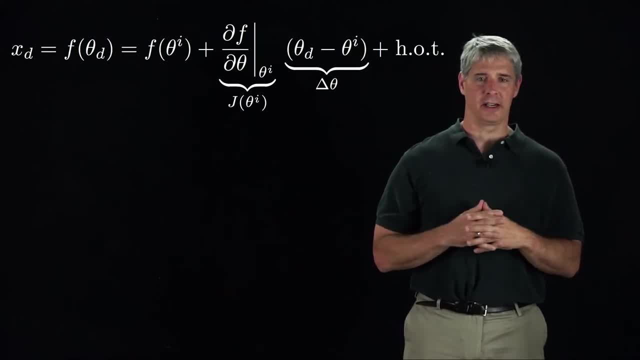 plus the Jacobian of f, evaluated at theta i times delta theta plus higher-order terms. If we ignore the higher-order terms, this simplifies to xd minus xd minus f of theta i equals j of theta i times delta theta. We can solve for delta theta as j inverse times xd minus f of theta i. 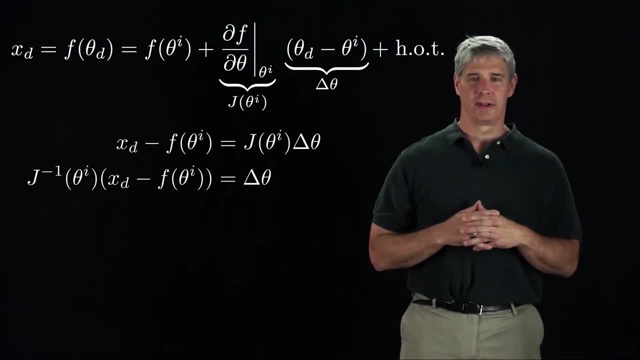 Of course, this only works if J is invertible. If J is not invertible, because it is not square, because the robot is at a singularity, we need a different way to calculate delta theta. Let's rewrite the equation we are trying to solve and number it 1.. 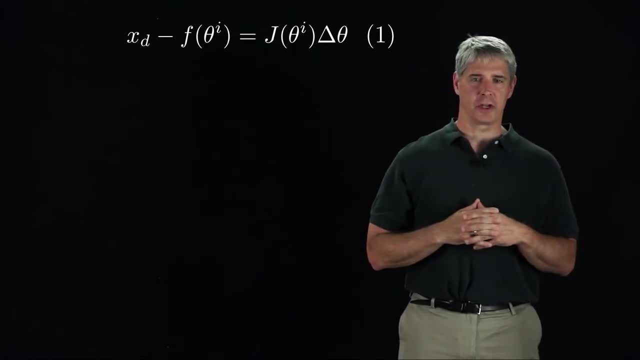 Instead of pre-multiplying both sides by J inverse, we could pre-multiply by the pseudo-inverse of J. The pseudo-inverse reduces to the matrix inverse in the case that J is invertible, but it can also be calculated for non-square and singular matrices. 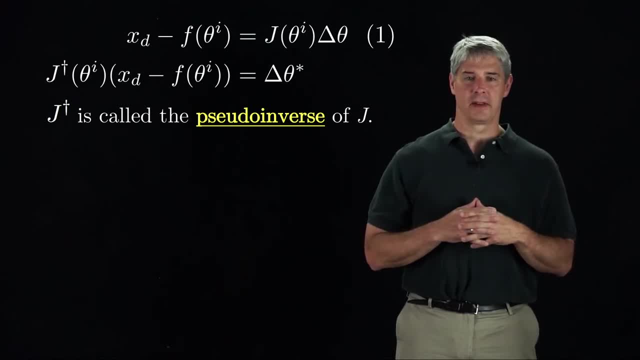 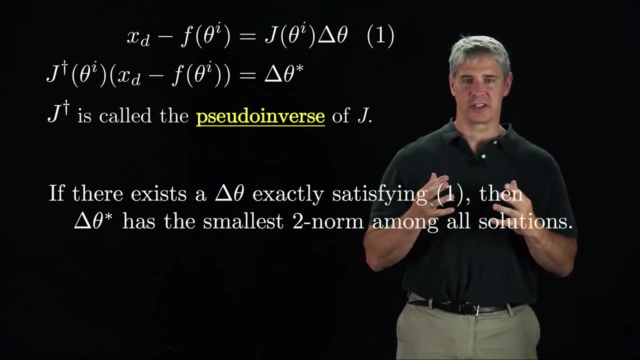 The pseudo-inverse has the following nice properties: If there exists more than one solution exactly satisfying equation 1, for instance if the robot is redundant, then the pseudo-inverse finds a solution- vector- theta star- that has the smallest length amongst all solutions. In other words, the change in joint values is as small as possible while still satisfying equation 1.. 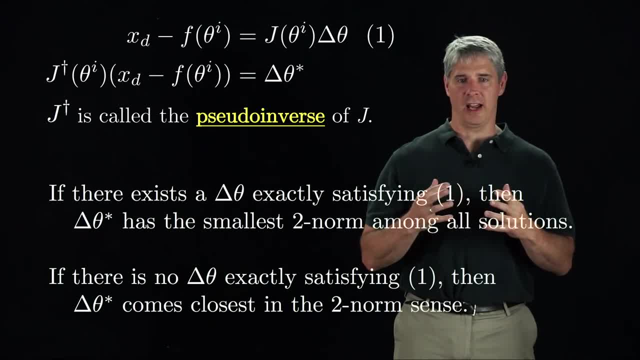 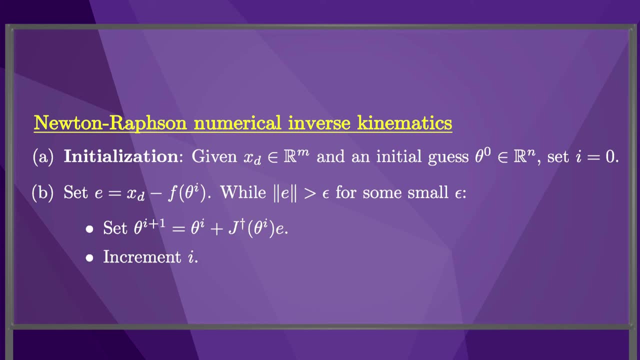 On the other hand, if the robot is at a singularity, if it does not have enough joints to exactly satisfy equation 1, then theta star, calculated by the pseudo-inverse, is one that minimizes the error in satisfying equation 1.. We can now state the Newton-Raphson numerical inverse kinematics algorithm.